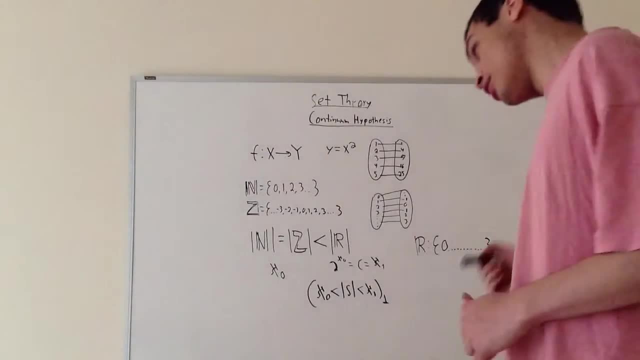 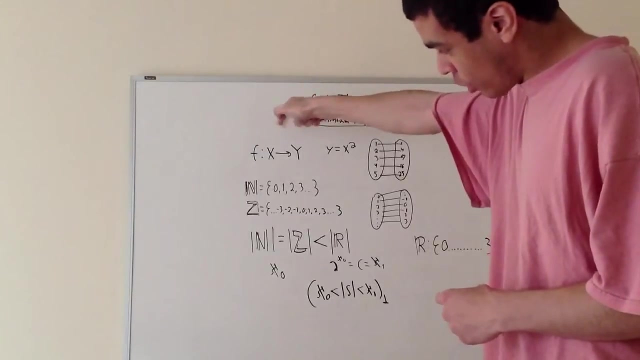 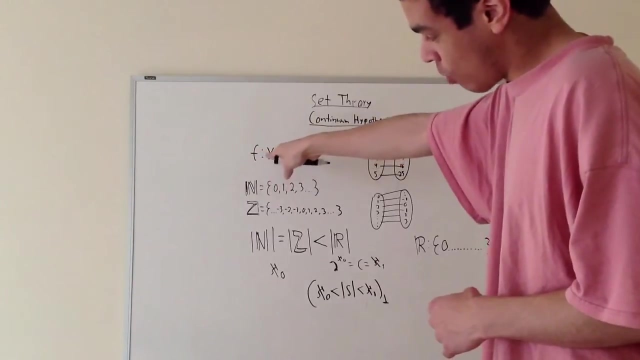 Alright, so this will be my video on the continuum hypothesis and basically I said in my last video that I'm going to show you why the naturals have the same amount of elements as the integers, and you know that's weird, but that's what's going on, So, basically. so, before I get into that here, I've written an important concept that we need to have down before I go forward. This is: if you're not familiar with this notation, this means that a function, f, you know, takes x and it maps it to y. You know it's really. just think of it as, like you know. 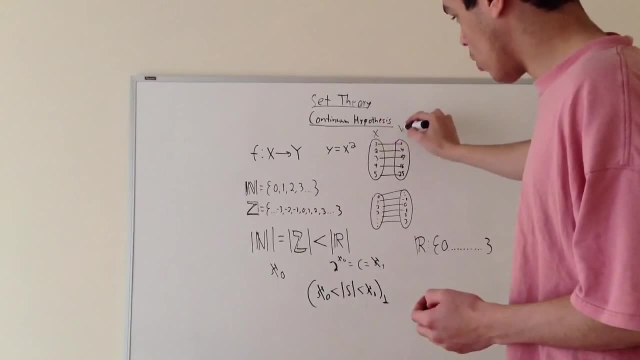 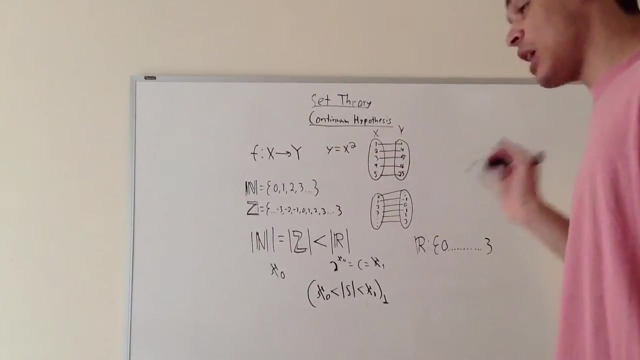 y equals x squared. you know from here, this is your x, this is your y. you know, this is your domain, that's your range and you have. you know 1, 1 squared is 1,. you know 2 squared is 4, so on and so forth. you know function: x maps to y, and that's really. you know what this is. And so, keeping that in mind, now, how does that business apply to infinite sets? Basically, here you know, the natural is like: you know 0,, 1,, 2, 3,. you know dot, dot, dot. and here you know integers: you know dot, dot, dot. negative 3, negative 2, negative 1,, 0,, 1,, 2, 3,, dot, dot, dot, all the way down. 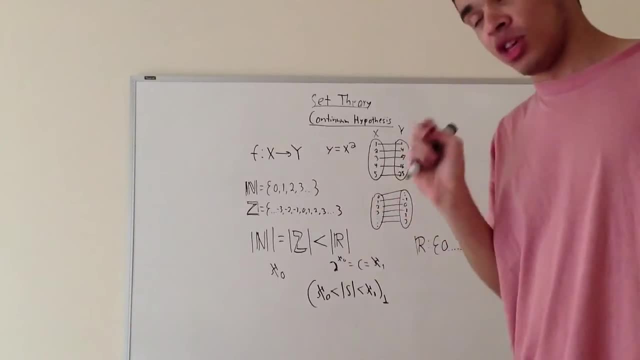 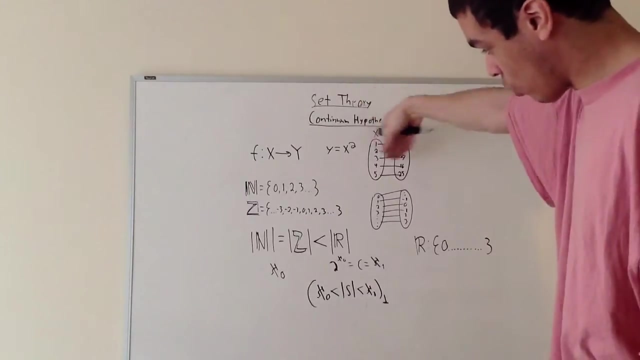 Now, the reason why they're equal is because I shouldn't say equal, I should say they have the same size. The reason why the sets have the same size is because two sets only have the same size if there's a bijection between them, which means that you can map exactly, you can really take this element and map it to one element. over here, There's always a 1 to 1 relationship. For each number, each x you give me, I can give you a y, And so that's a bijection or 1 to 1 relationship. and because and two sets are only equal if, or equal if, and only if, there's a bijection between them. 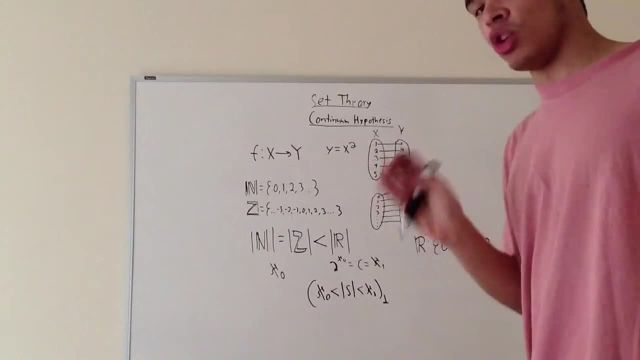 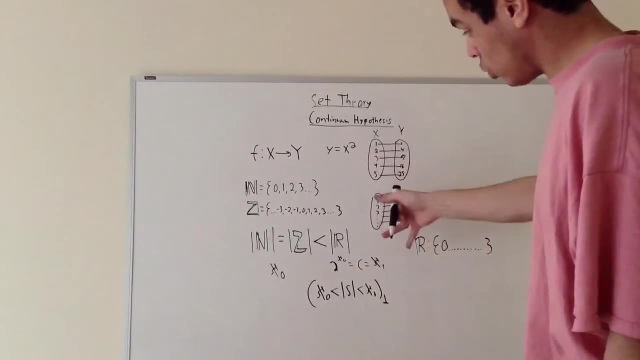 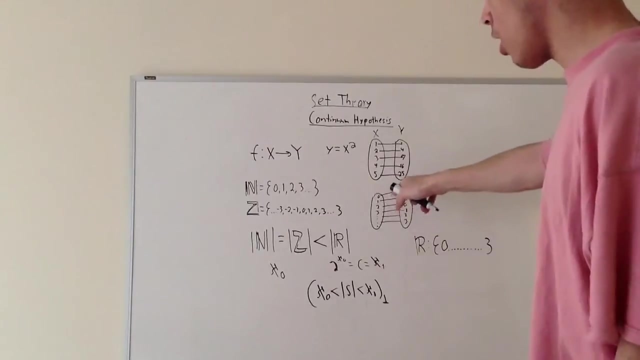 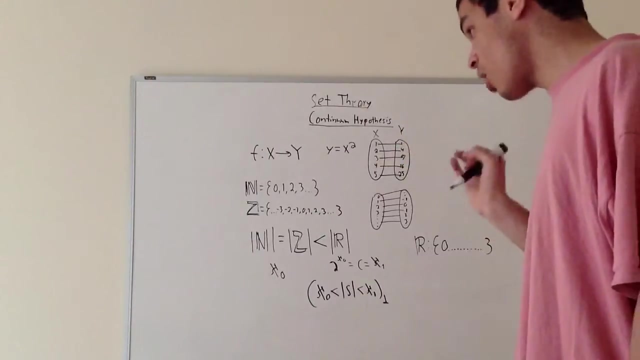 between the two elements And for the naturals and the integers there is a bijection. Here's why: because you can start with 0 and any integer you give me, no matter, you know what integer it is. I can take 0 and you know, say this: you know maps, maps over to whatever integer you give me And I can, you know, repeat that for 1 and negative, 1 and 0. Now if you took a subset of the naturals and a subset of the integers, like if I had, like you know, let's just say I took a subset of n here, like you know, 1,, 2,, 3, that would be a subset of n here. 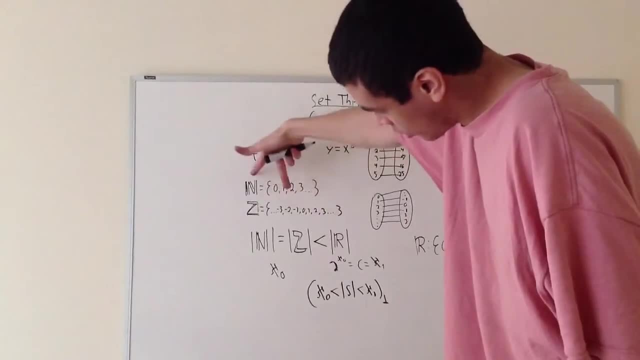 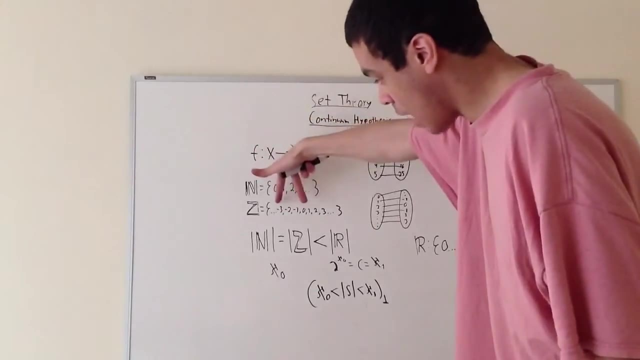 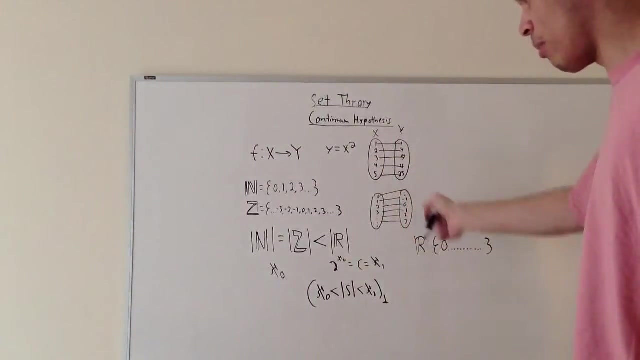 And here I took all these elements. Clearly, this subset is smaller than that one. That's because it's finite and I cannot. I cannot make a 1 to 1 relationship between 1, 2, 3 and 3, negative 2, 1, 0, 1, 2, 3.. Because it's infinite. I can keep going, I can go on and on and on, and I'll never run out of elements to map here. And a very important concept is because the reason why we can do that is because every single element, we know where the next one is. We know that. you know negative 3, the next one's going to be negative 2, the next one's going to be negative 1.. We know exactly what the next element is and because of that we can map. 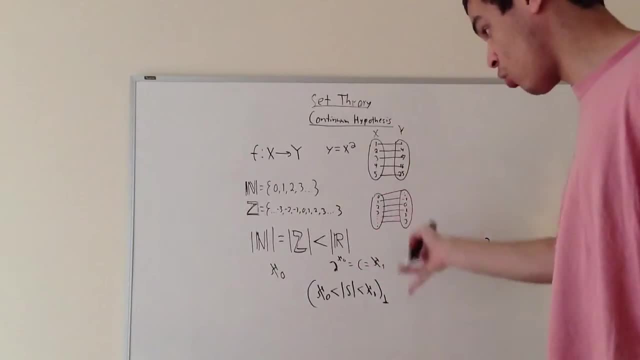 from one set to the other And because we can map, because there's a 1 to 1 mapping between the two of them. that's why they have the same size. Now, how does this apply to the real numbers? Basically, there's a mathematician in the last century- 20th, I think, 20th, 20th or late 19th- Geyer Cantor, And basically he was kind of the first one who studied infinite sets and cardinal and all that stuff And basically he kind of spent, like some, a lot of years in his later years. 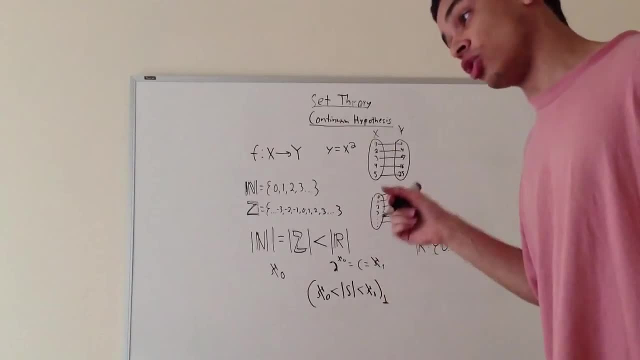 later life trying to prove the continuum hypothesis. And actually the continuum hypothesis actually cannot be proven true or false, And that is a concept which I. another concept which I'll revisit later when I talk about this is a Melo-Frank-Kell axioms, But basically, 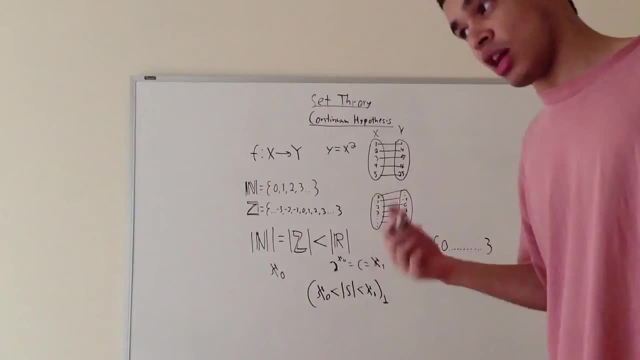 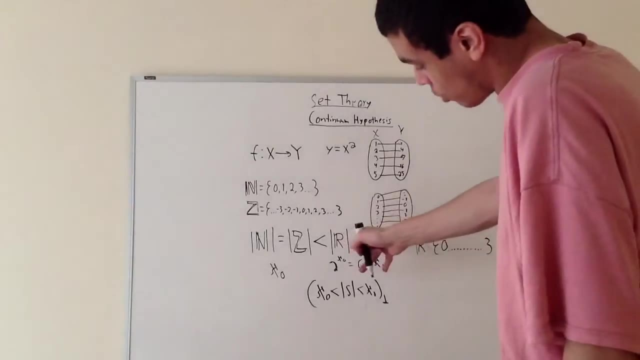 he kind of went. he kind of went nuts trying to prove it and he couldn't prove it and I think he actually killed himself That was. that's an interesting story, But anyways. so the real numbers is the reason and the real numbers have a different cardinality. 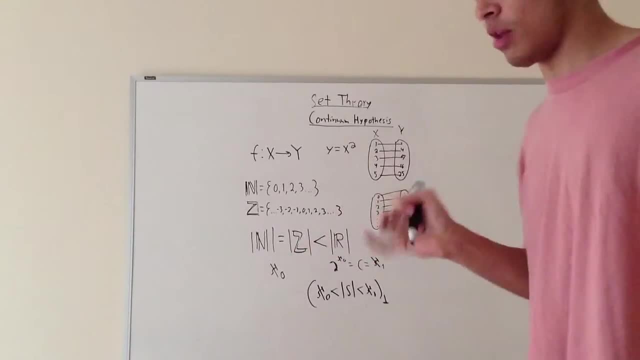 than the natural numbers. So the real numbers have a different cardinality than the natural integers. They actually have what's called an uncountably infinite amount of elements. And why is that? Because for the real number, let's say: I start with 0, right, And we don't. 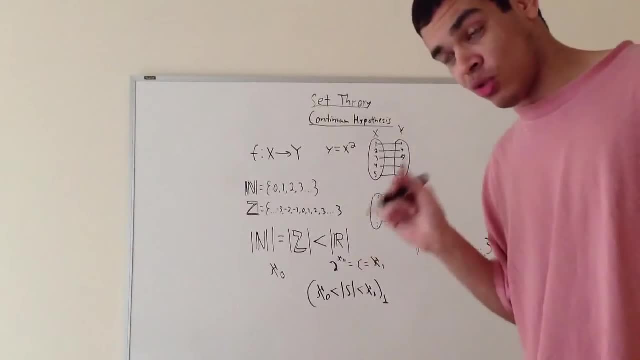 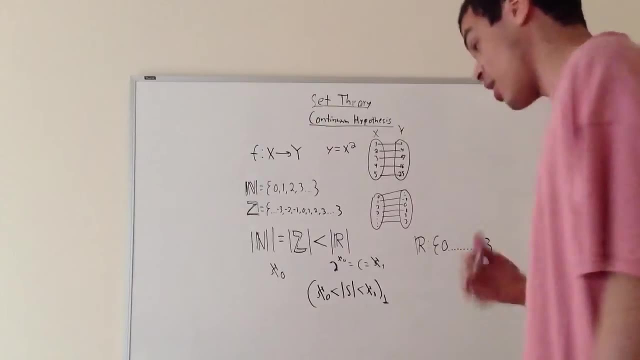 know what the next element is, And because I can just do 0.01,, I can do 0.01,, I can do 0.0000001 and go on indefinitely. And because we don't know where the next element is. because 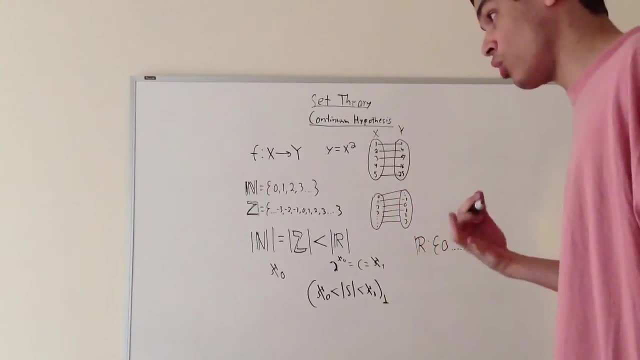 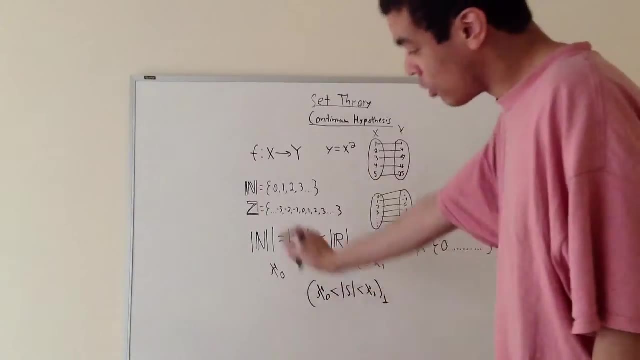 the next element goes on and on and on. we don't, we don't really have a way to, we can't, we can't strictly specify what the element is And, and because of that we don't know that We cannot map the naturals. we cannot map the naturals or the integers to the reals. 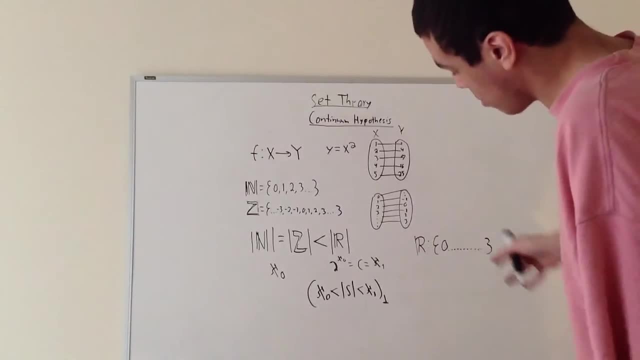 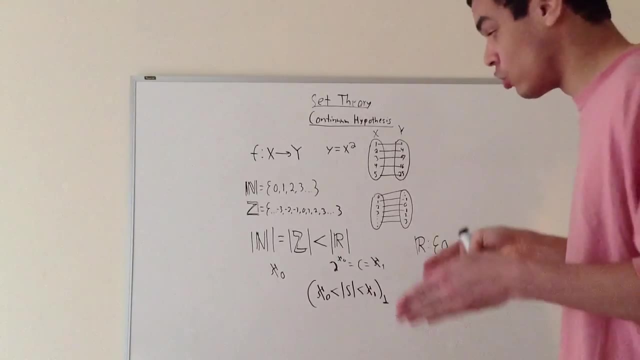 and have a one-to-one relationship. We just don't know what that is. And- and this is what's really interesting- is that the spacing between each real number is like, you know, the, the amount of like, if we had 0 and 1 and we wanted to know, and let's say you, 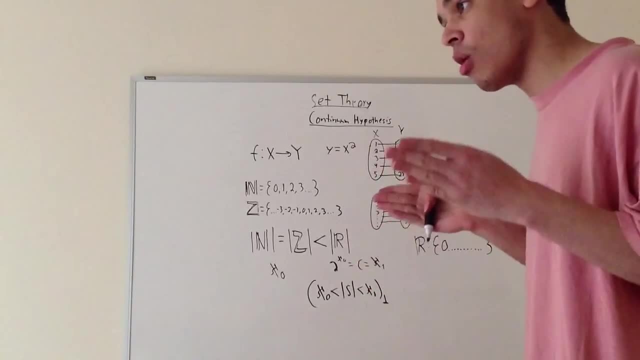 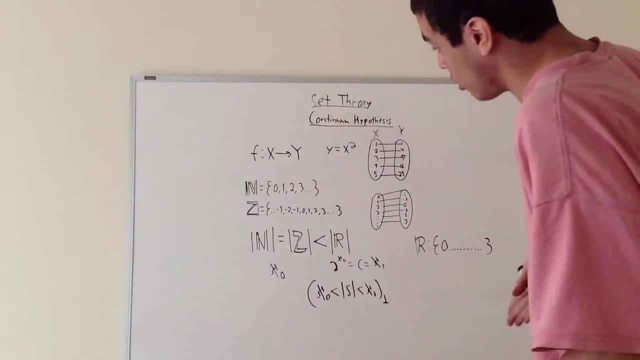 know, the amount of reals between 0 and 1 is actually more than the entire set of naturals and integers, which I think is a really counterintuitive thing. If you study set theory long enough, that's really kind of. that's kind of a weird, weird. 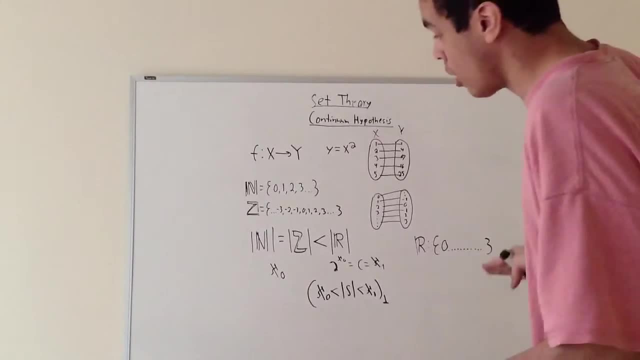 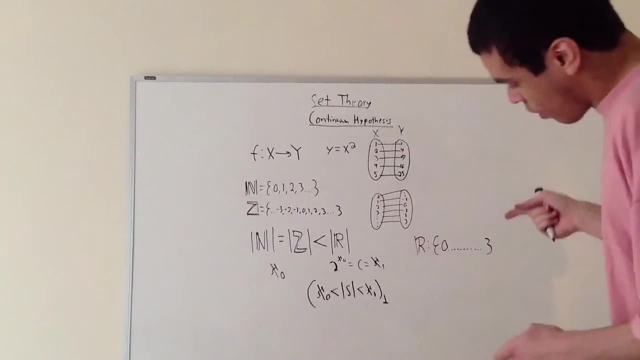 concept And maybe I probably should have done this video, maybe towards end of set theory playlists, but really the the stuff I talked about earlier is enough to kind of understand this, But basically. so this is like that's a really weird thing to think about, because 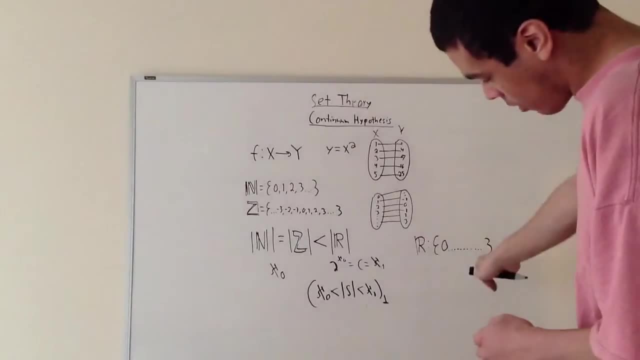 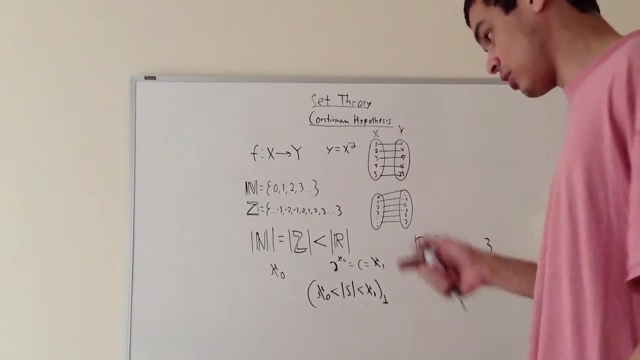 like you know. this is why it's uncountably infinite, Because we just don't know where the next element in the set is to be to. that's really why we don't know, And so, Gierer-Kantor, his hypothesis is that there is a. there is actually. 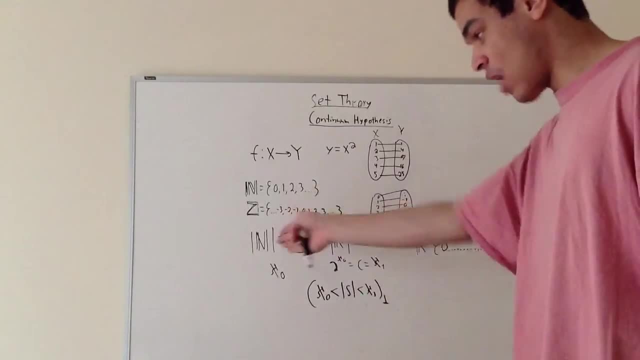 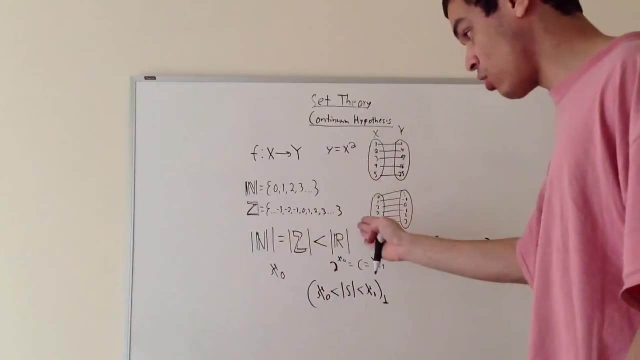 no set that has a cardinality between the naturals and the reals, which means that it's either natural whether the size of the set is either the size of the naturals or it's the size of the reals, and there's nothing in between them. There's no size that exists. 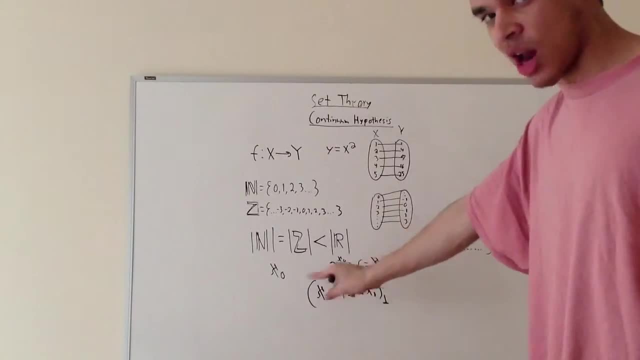 between them. And that's, you know, can be written like this: you know all if not, which is the cardinality of naturals. There's no set, that's you know greater than that, but less than the reals. That, and this is a little upside down, T means false, And so, basically, 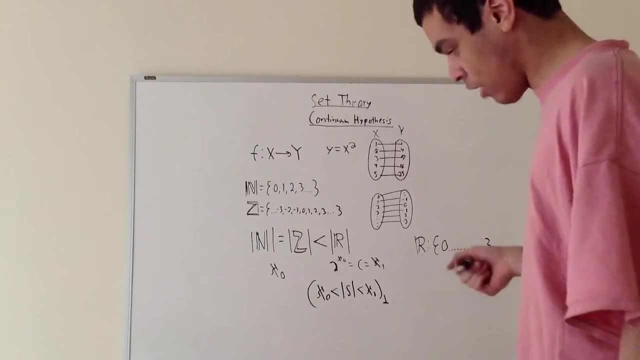 that is the continuum of problems And this actually can be generalized kind of more. That that you know really. actually, before I even get into that, I should say that all if one is, you know there's a couple of ways to write that You can write, you know, C. 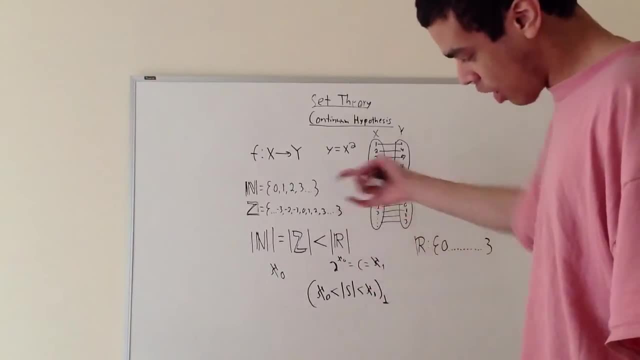 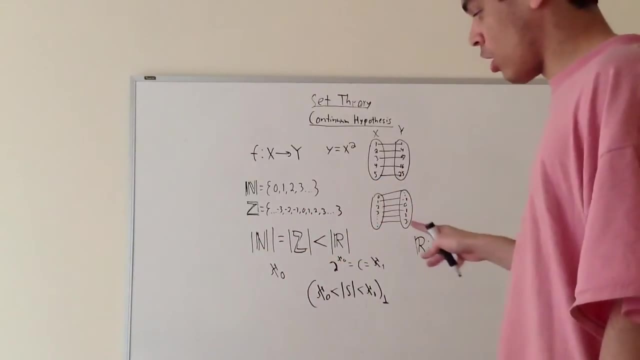 which means cardinality, continuum, Or you can also write this, as you know, two to the all, if not, And really this is like the idea that the reals are the power sets of the naturals, And so, basically, you know another interesting property- well, not really property, but kind. 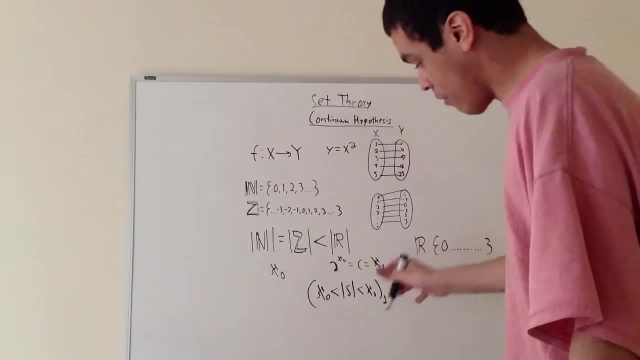 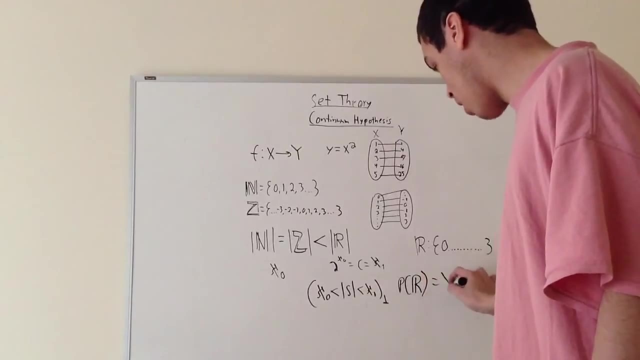 of idea from the that stems from the continuum of problems is that you can have that if you have like a higher cardinality, like if you wanted to take a higher cardinality, take a power set of the reals that would be equal to all of two, which is the next. 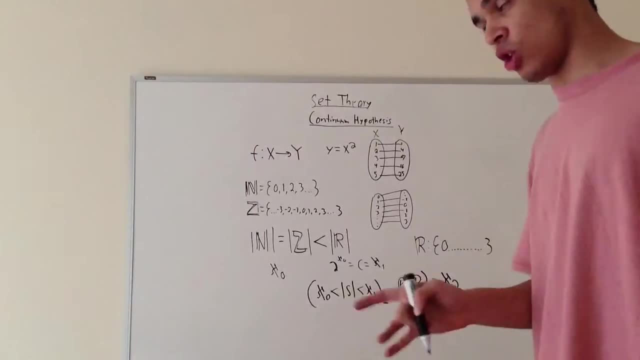 uncountable, uncountably infinite. cardinal, That's the term. Cardinals are basically, like you know, all of all of, not all of one, so on and so forth. They're kind of like degrees in infinity, Because basically, when people say infinity, well, when lay people say infinity. 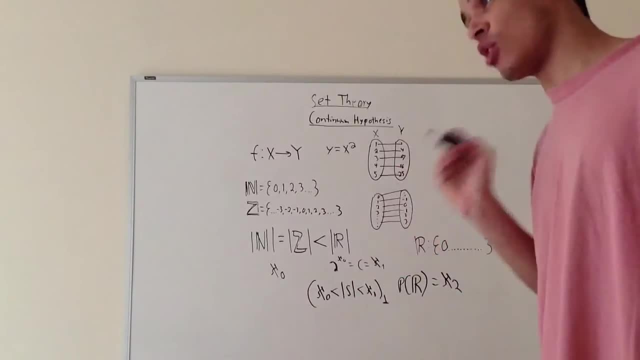 they don't really. they do not specify that they're actually, they don't really know that there are different levels of infinity. Infinity, when you say infinity, that can mean several different things, as I just kind of, you know, been going on for a while, So you know. 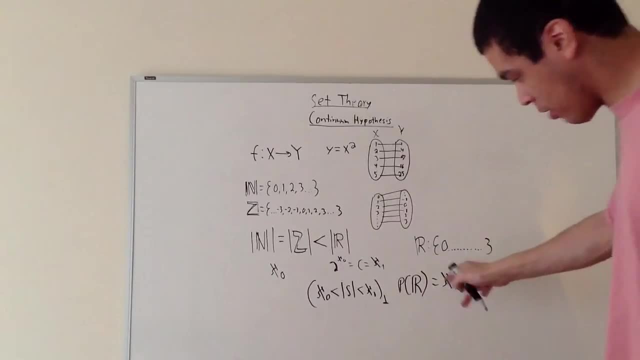 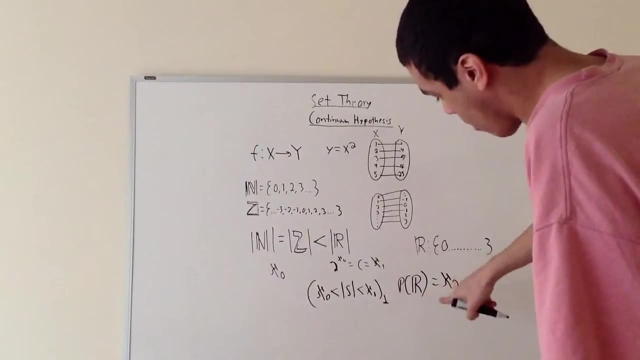 on and on about. So, basically, the power set of the reals is cardinally all of two, and there's actually there's no cardinality that exists between all of one and all of two, And and so you've got all of three, which is, like you know, all of three would. 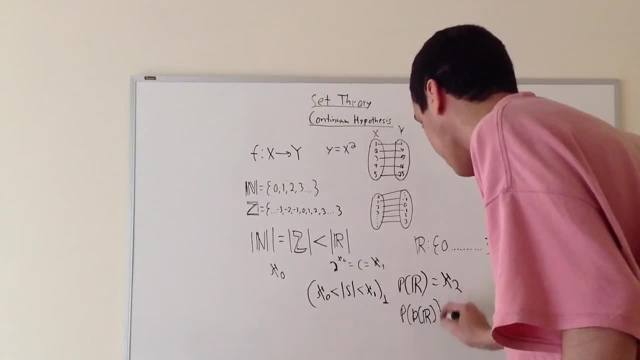 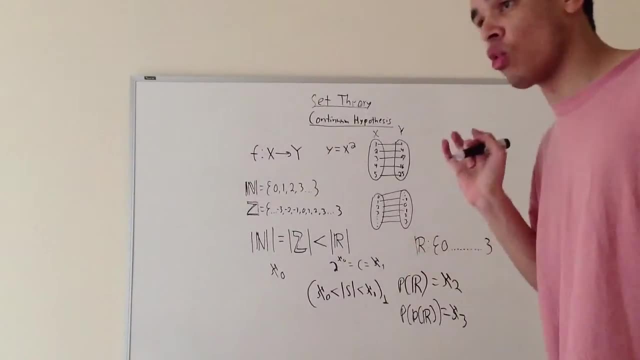 be the power set of the power set of the reals. That's and, and, and. actually, before I even like go any further, that's a really weird thing to think about, because what exactly would the power set of the reals be and what exactly would the power set of the power set? 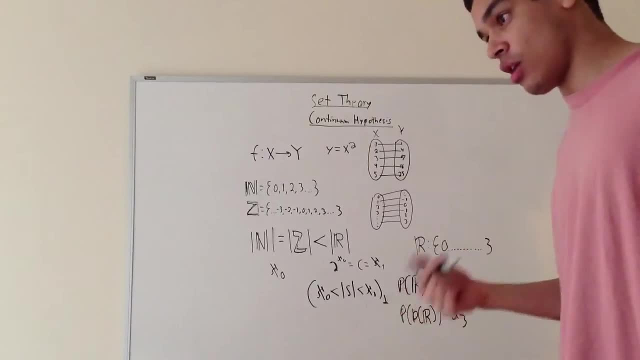 of the reals be be like. you know the amount of elements in that set are just it's greater, but you know what will those numbers really be like? that's an interesting thing to think about and I really like it's kind of hard. it's kind of hard to really understand what that. 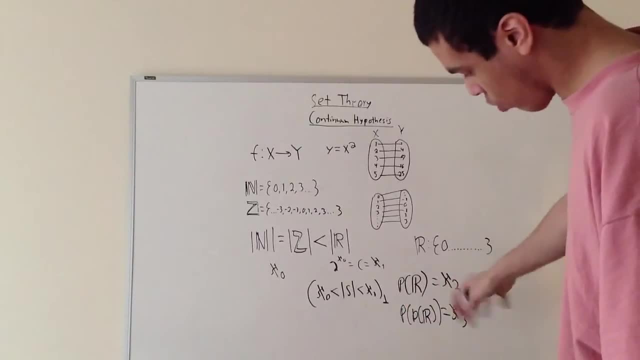 really means and basically that's kind of what the content hypothesis is all saying. this is like the more. I think this is called the generalized version. I'm not really sure if that's like the prop. I don't think that's really exactly what it is. maybe it is maybe. 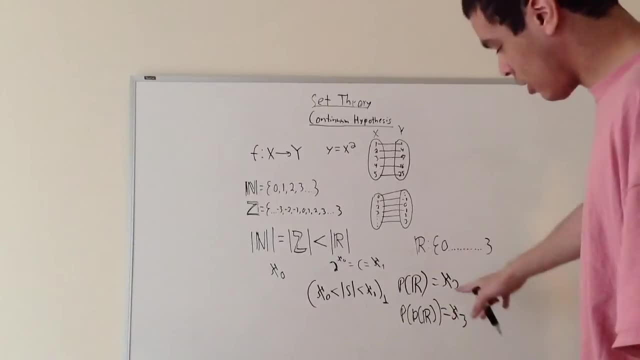 it isn't. I don't remember. it's been a while since I've like looked at that, but basically, um, the idea is the same. what I'm saying here is still true that the idea is that the cardinalities there's Aleph 2, Aleph 3, that's the next cardinal. there's nothing. 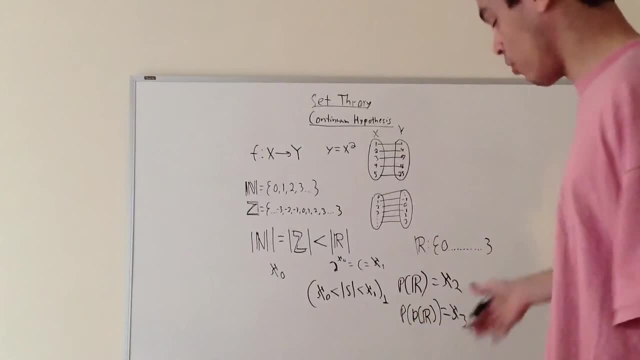 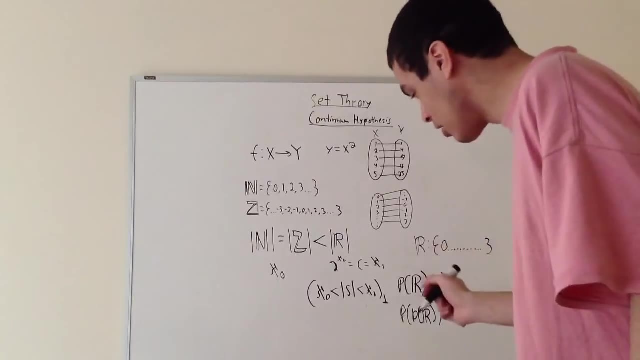 in between any of these cardinals, any set you can come up with. they either have this cardinality or that cardinality, nothing like you know, Aleph 2.5,, nothing like that, and so, um, basically, and you can kind of like, of course you know whenever you write Aleph. 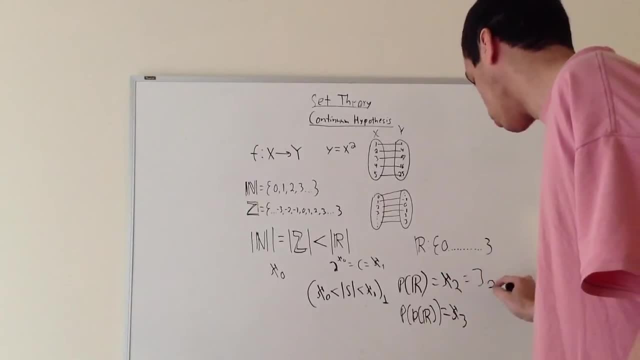 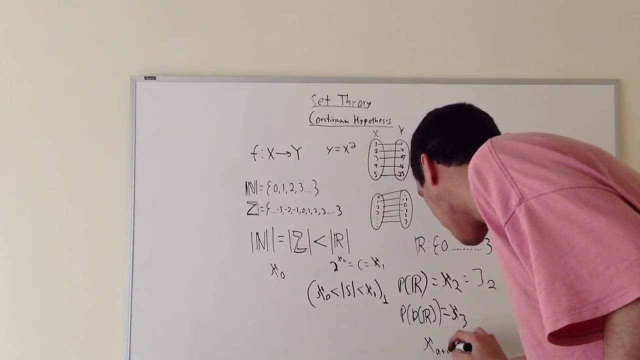 you can also write Beth, that's just an you know, which is like this letter, which is an alternative, and basically in general, like you know, when you have a cardinal, Aleph A plus 1, that's just equal to um, the power set of the previous cardinal, always that's. 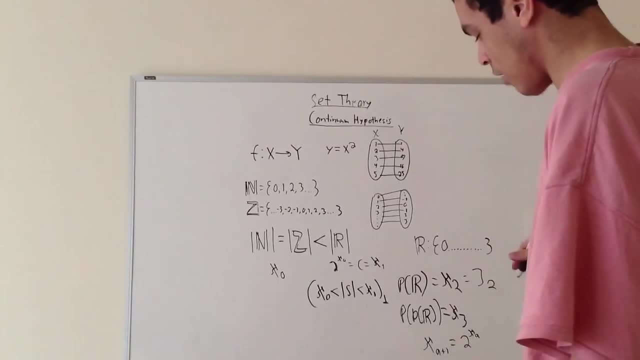 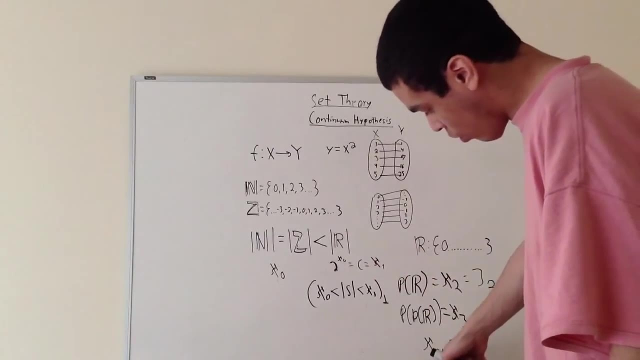 always the case, um and and so that's that's kind of the idea. and also now here's where it's really interesting, because what if, what if this A down here, what if the what if this uh index here is actually like this? what if it's like this: you have Aleph and 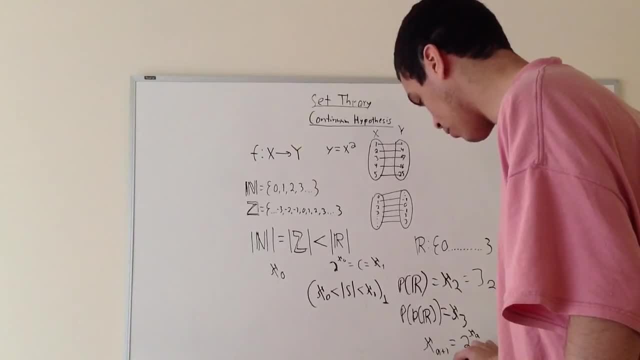 then you have uh, I guess, um, I guess Aleph naught Uh. so basically that's the idea. Uh, so basically that's the idea. That means that you have a countably infinite amount of uh cardinals here. 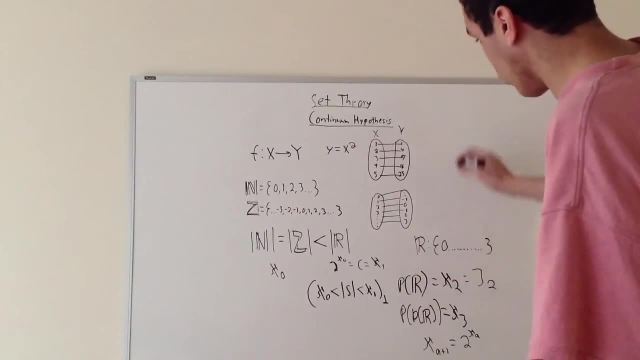 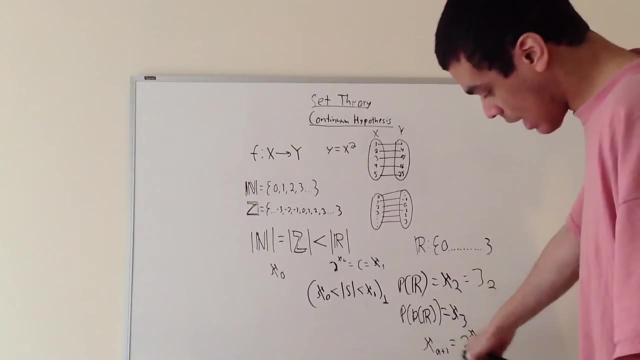 So you basically, like you know you have, you basically take a. uh, let's just say, we take another set. um, actually I won't even like get into that. Basically, the idea here is: you can keep adding, adding, adding and eventually, uh, there's. 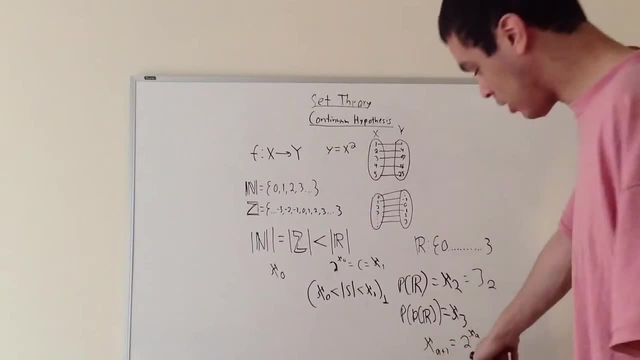 a point where, uh, well, shouldn't say I shouldn't say that, but basically, there there is a, there is a um, it is well-defined, it is the. it is the fine set theory that you can have a countably infinite amount of cardinals. 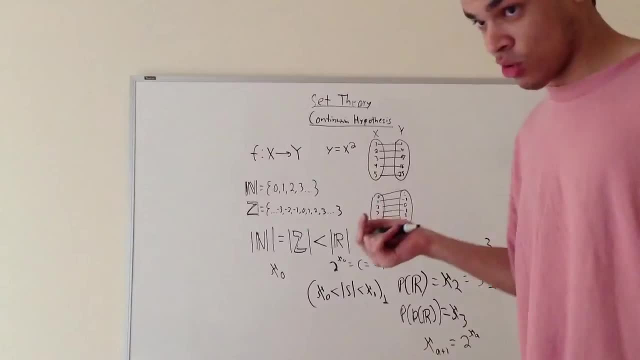 And that gets into, like you know, uh you know ordinals and uh you know, there's actually like a whole system of uh arithmetic and like you know, uh multiplication, all. 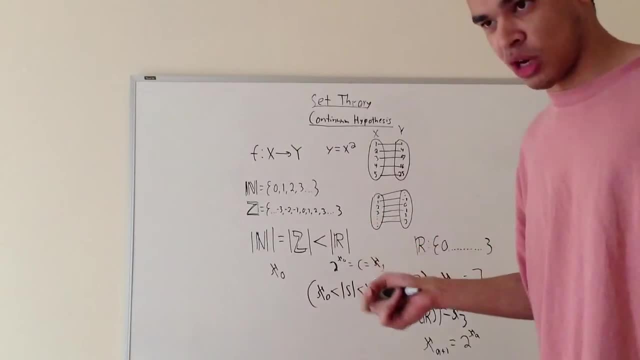 that stuff, that um is, uh, that is that's being, that's being studied right now. Uh, basically, it's kind of like you know what I like to call the search for the highest infinity. like you know what, exactly? how high can we go? 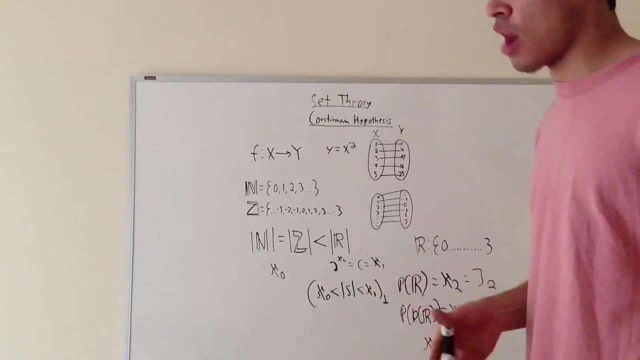 That's kind of any reason to do. the content policies now, I think, is kind of based on that, like how high can we go, And so this is kind of like you know, uh, where that kind of idea steps from. 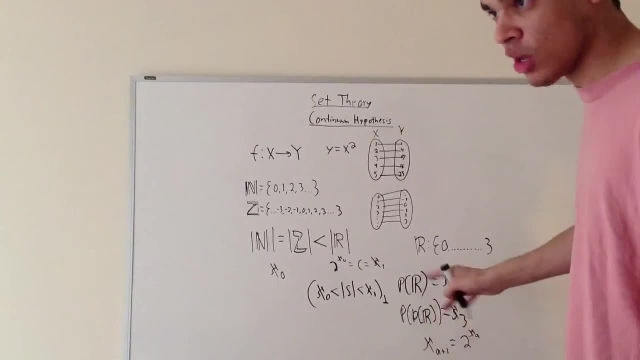 What, what, what would be the highest, The highest possible cardinal ordinal that we can possibly construct and, um, you know, uh, and it still be still makes sense, Like what it doesn't make mathematical sense. 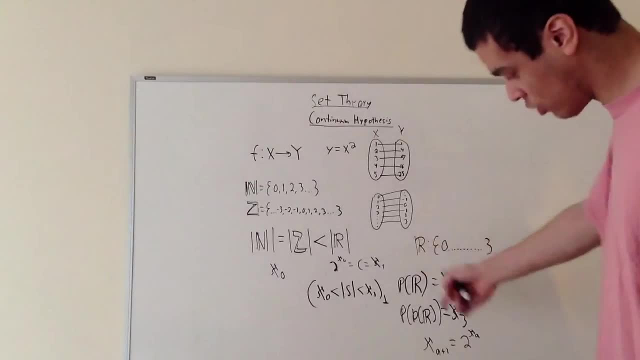 Like these make mathematical sense. They're well defined. they're defined, you know, this is the power set, that's what it equals to, What's the highest ordinal that we can, or cardinal cardinal that we can construct, that will have the um that can be well defined. 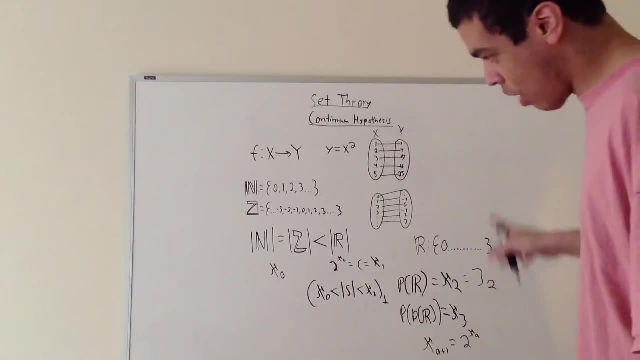 And that's really what the content hypothesis is really all saying. And so in the next video I will be doing um, I'll start talking about the uh Zermelo and Frank Kell. uh um axioms.